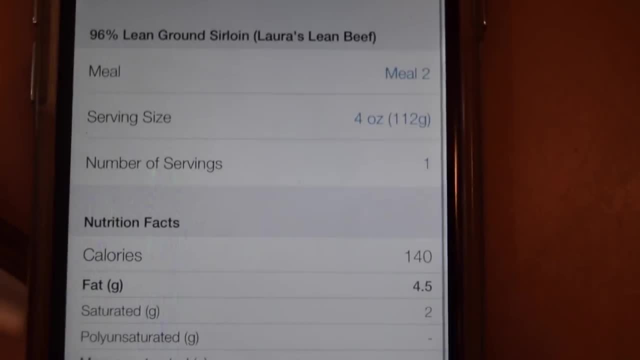 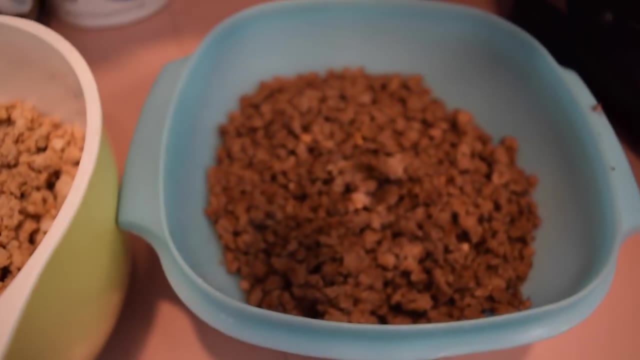 protein and this is the nutrition data that comes for four ounces just labeled raw beef based on the 3 year old before that. but the raw beef is specifically on the package. but you have to keep in mind, guys, that is the nutrition data for the raw weight. the nutrition data on the package will always be the raw weight. 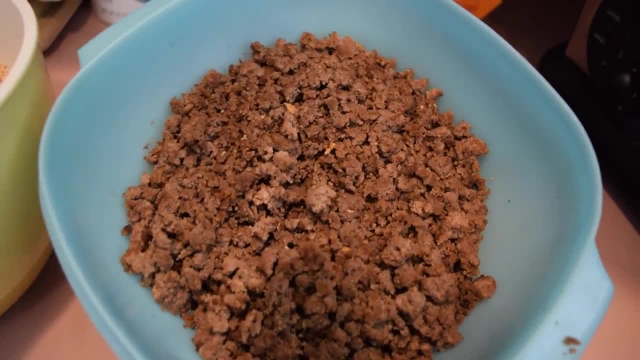 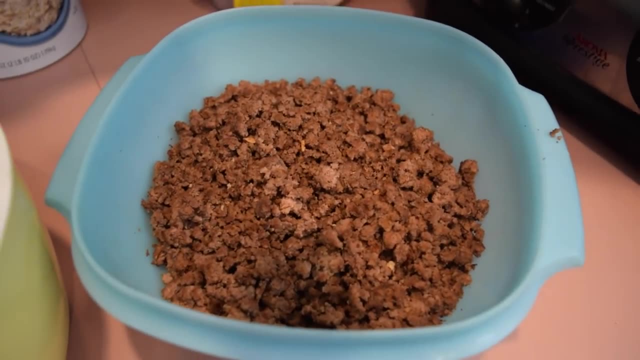 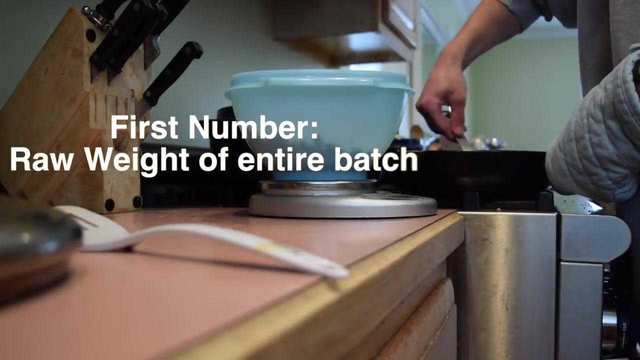 after I cook it. we already saw that it weighs about 10 ounces less, so how do we track it accurately? it's actually really simple to figure out how much 4 ounces raw weighs cooked. all you need is three numbers. the first number is the raw weight, which we already got when we weighed this beef before preparing it. 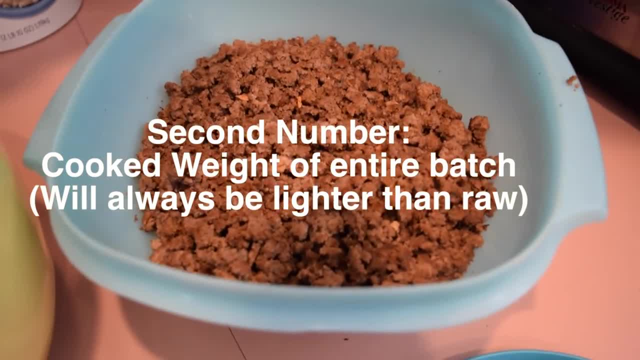 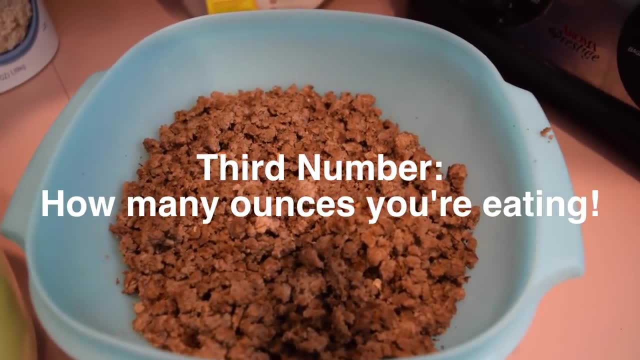 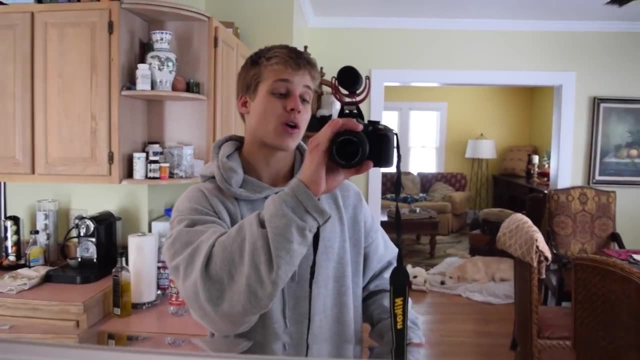 the second number is the cooked weight which we took afterwards and you saw was 21.9 ounces. and the third weight is whatever you want. do you want two ounces of beef? do you want four ounces? do you want eight ounces? it's whatever you want to eat. for argument's sake, let's say you want four ounces of this ground beef in. 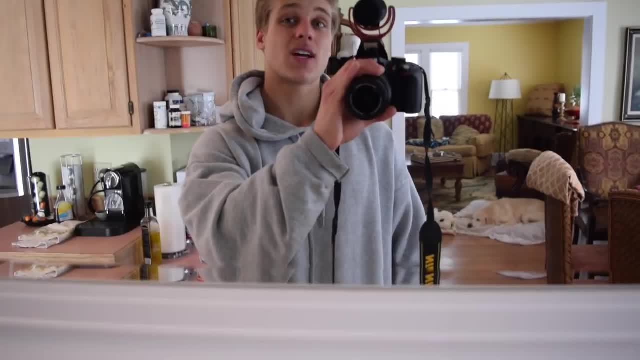 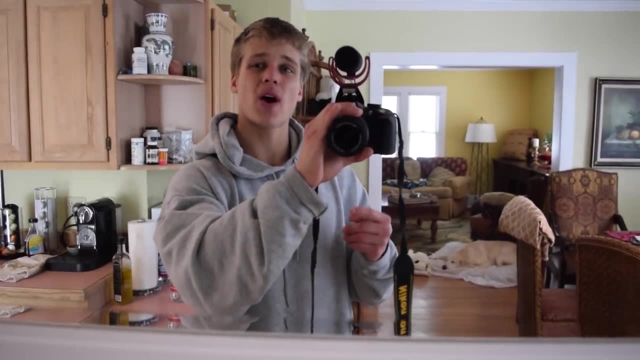 your next meal, four ounces. according to that nutrition label is 4.5 fat and 23 grams of protein, but that's four ounces raw. so what do you weigh out when you already have all of the beef cooked up? this is really how simple it is, guys. as you see, we had 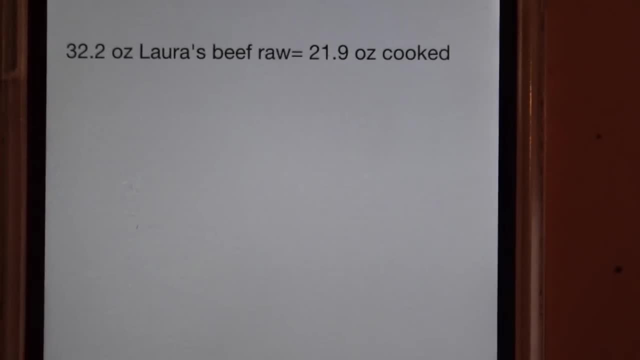 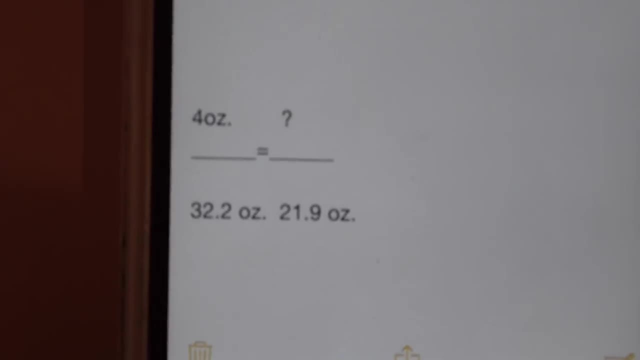 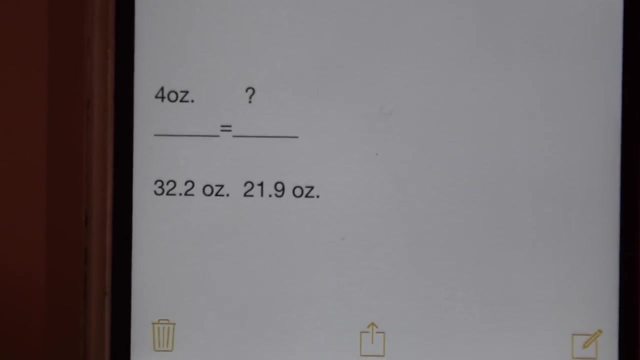 32.2 ounces of the beef raw, and then we cooked it and it weighed 21.9 ounces. so all we do is we set up a proportion. check this out: four ounces raw over the entire batch. raw equals question mark over the entire batch cooked. as you see, 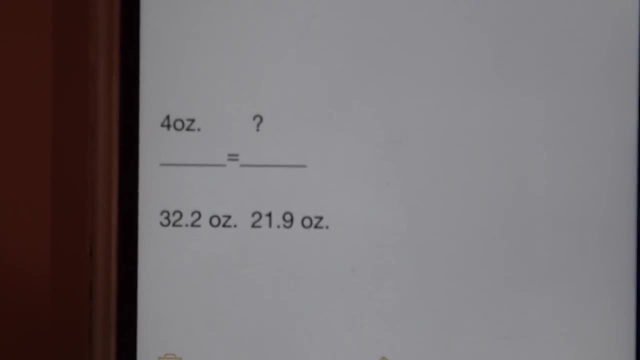 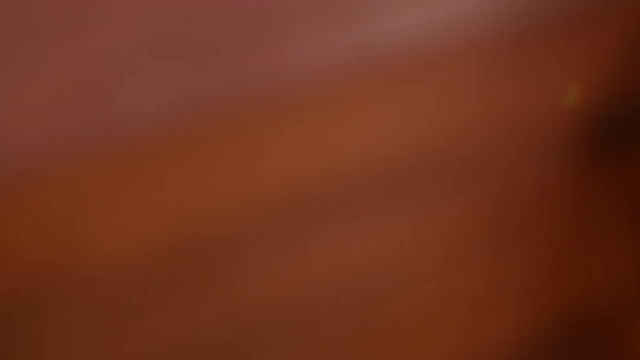 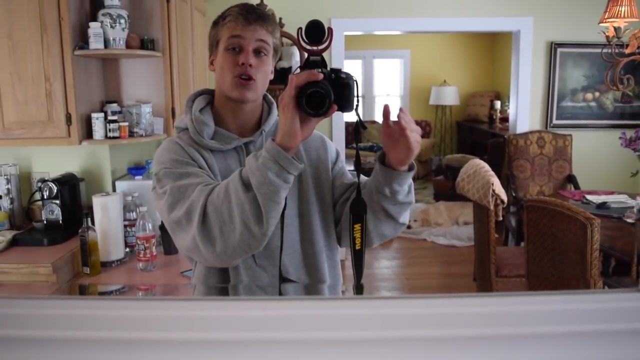 the 32.2 ounces is the raw weight and that 21.9 ounces is just the cooked weight. after calculating this, we get 2.7 ounces cooked. so four ounces of this raw beef is 2.7 ounces if I were to weigh it out cooked, and that's what I'll do if I want. four ounces. if I want eight ounces, it's just twice that, so I believe that's 5.4 ounces cooked and so on. it's a really simple way to just account for the water that's lost in the meat after cooking it and get the correct amount of protein. 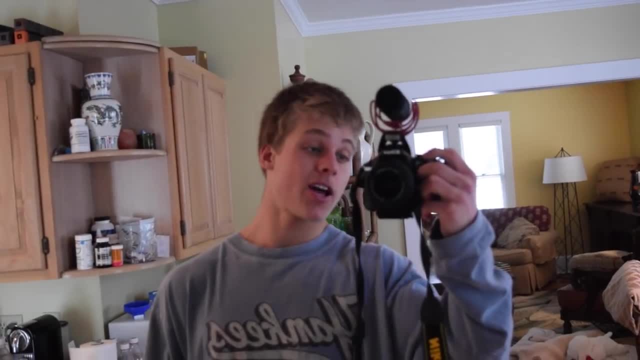 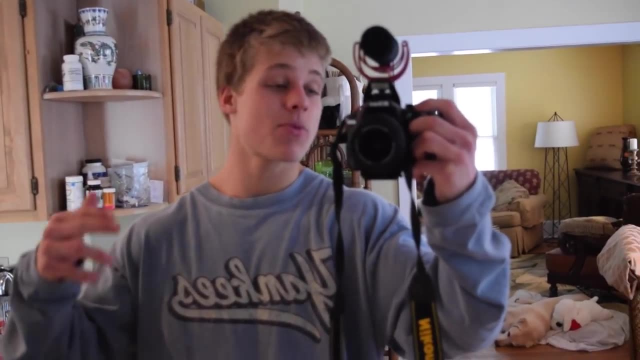 that you need in each of your meals. it is a little bit later now. as you see, I'm in a different shirt. I showered up and I'm about to do some homework, but I just want to get that quick tip out for you guys. keep in mind, as I said before, if